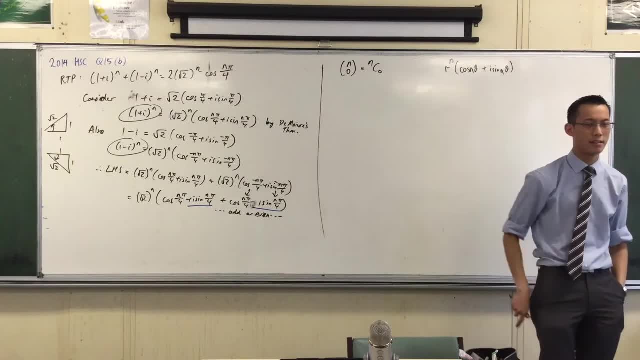 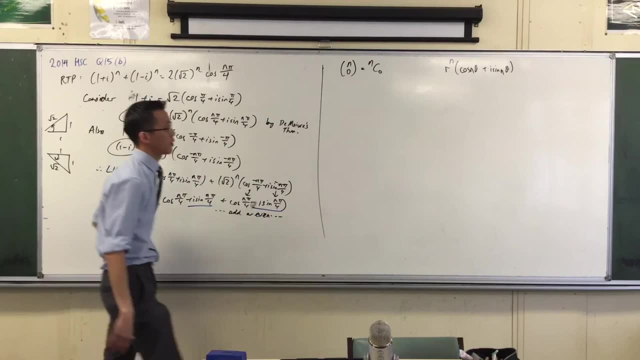 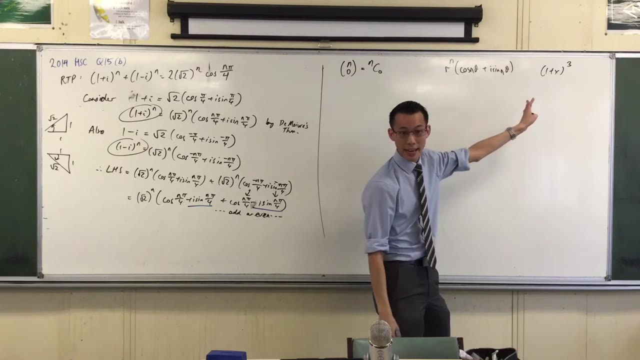 You go from zero all the way up until n. Why would you go all the way up until n? Let's think about it this way: If I gave you, you know, 1 plus x, cubed right, The binomial coefficients that you're going to get out of that from Pascal's triangle are going to be n naught. 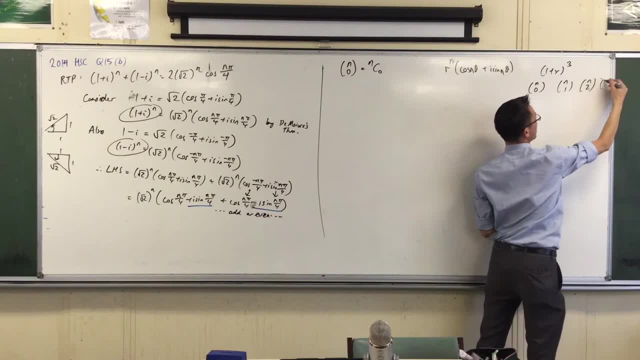 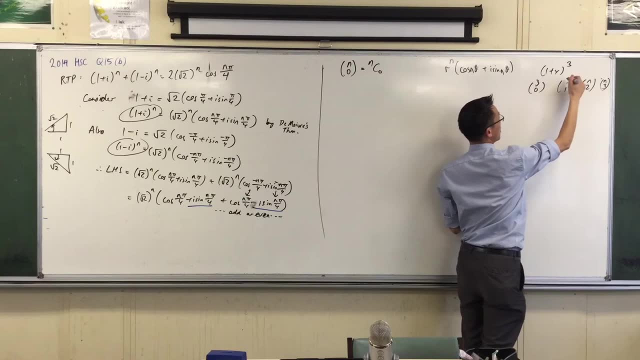 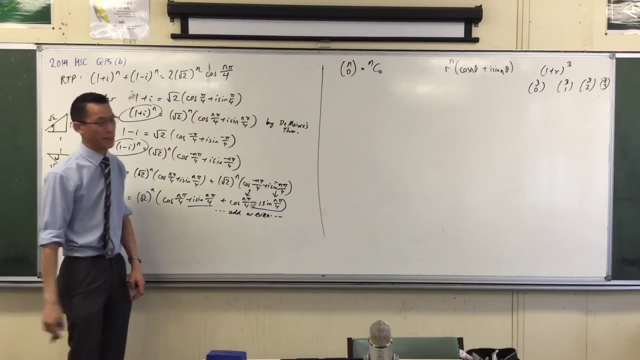 and then n1,, and then n2,, and then you'll end with n, So n is 3, right, Where n actually happens to be 3, in this case right, 3, 3, 3, 3.. Because of course you can't have 3c4, because, like, how can you choose 4 objects out of 3 things? okay, 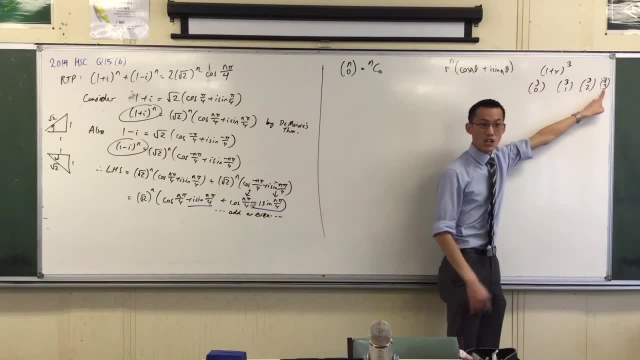 We have 3s all the way at the top and 3 at the end. because? because the power is 3.. Power is 3.. Here I've got n's up the top, a whole bunch of them. Why would I have n's up the top? 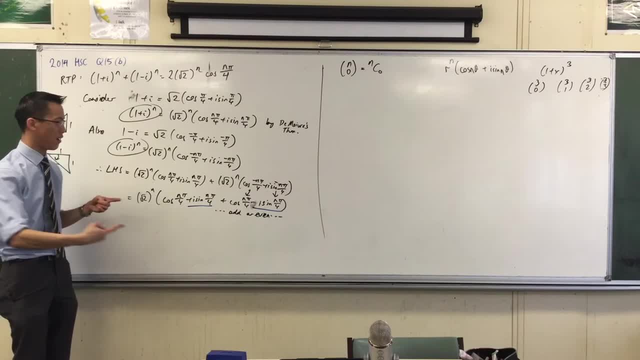 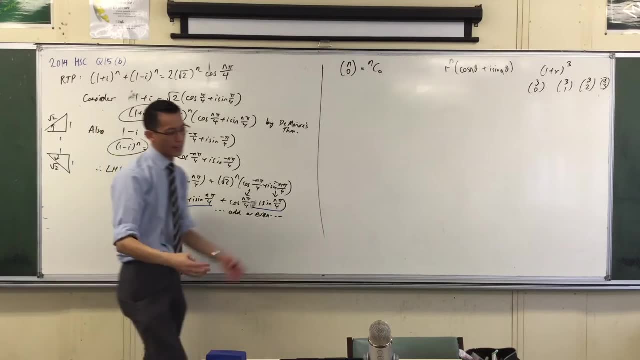 Because I'm expanding something to the power of n. Yes, Okay, Now, where a lot of students sort of fell down is they felt like- and I hope you recognize this is something we need to overcome- You look at a question and you classify it and you think, oh, this is a question about that. 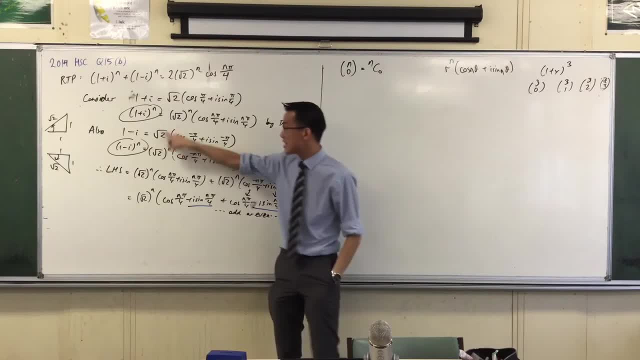 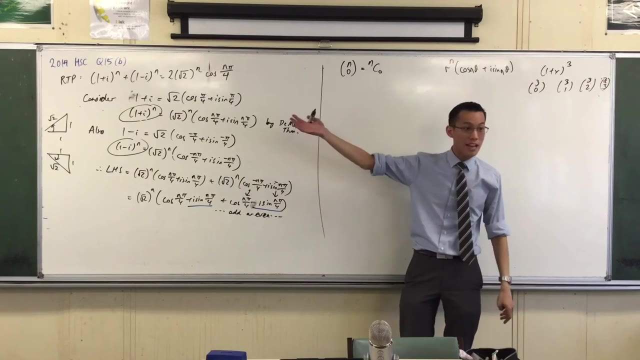 But these are clearly linked right. So you should see these n's and think, oh, I can treat this not like I can't just turn this into from rectangular form into polar form. I can treat this as Just a regular binomial expansion. It's just that that second thing happens to be imaginary, okay. 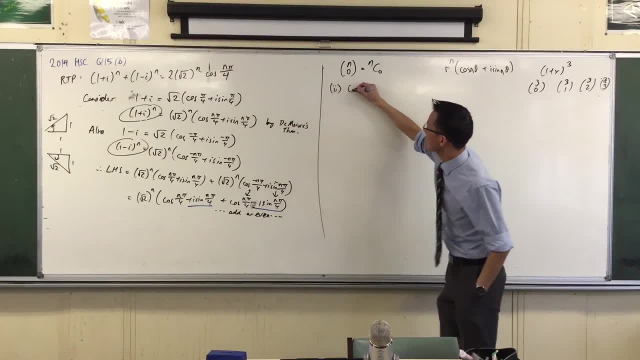 So let's do that right. This is part 2.. Consider: I considered this before and I did de Moivre's theorem on it, right, But now I'm going to do binomial theorem on it, okay, So what will the very first term be? 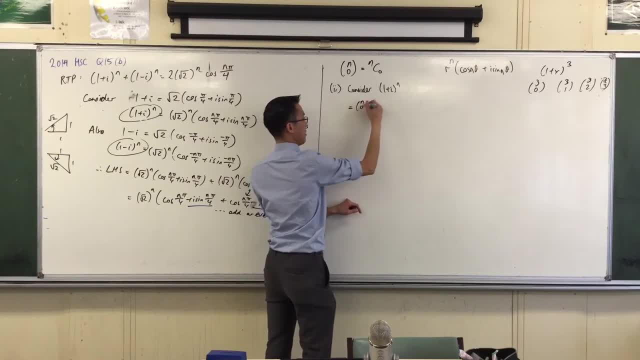 n 0.. Actually, I'm going to write this on the next line: n 0.. The next one's going to be n 1.. n 1.. But now that I get to the next bit, an. i comes along for the ride. 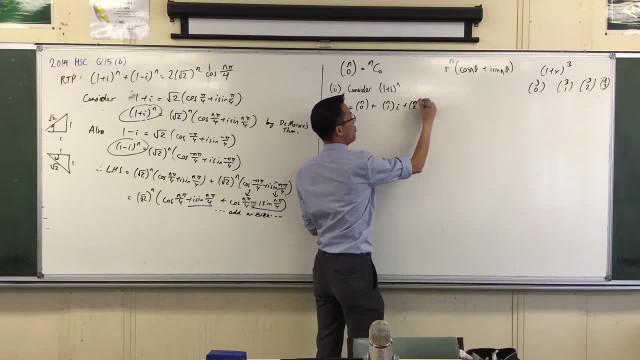 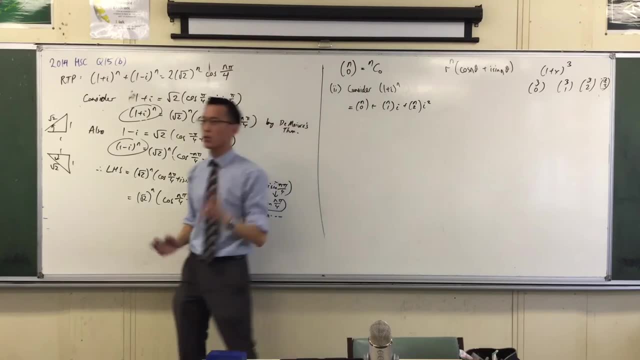 Do you agree with that? i, And then n 2. And I'm going to have um. I'm going to have two i's, aren't I? i squared. Okay now, usually to establish a pattern, three terms is enough, right. 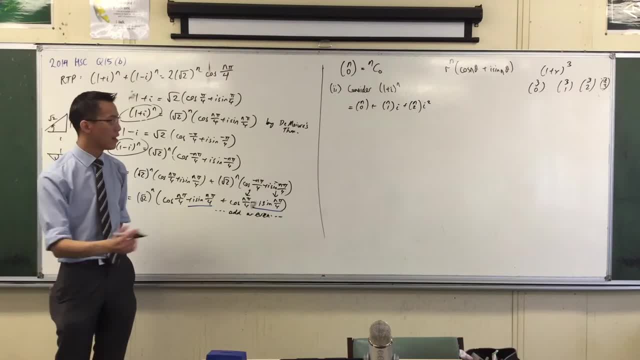 Like, if you get three terms of an AP or a GP, you're like I know everything about this. now, okay, For reasons that will become clear shortly, I'm going to put a couple of extra terms on right. I'm going to go n 3.. 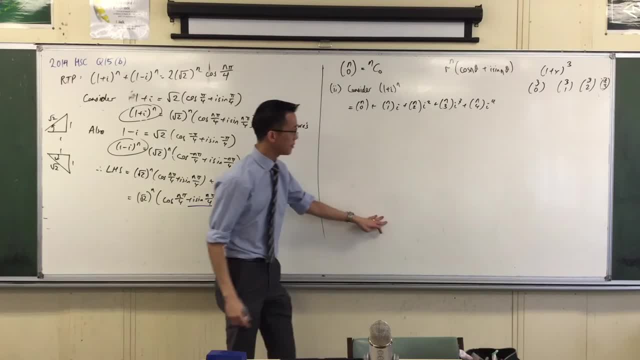 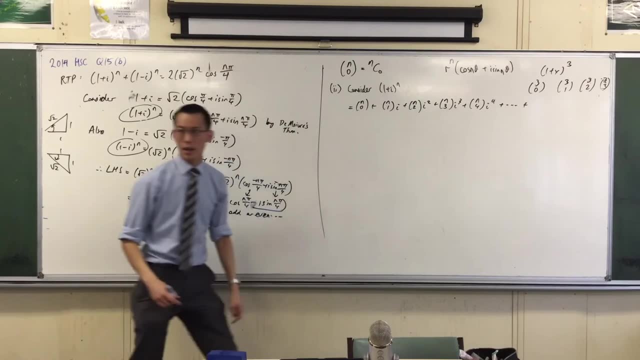 And n 4.. I think that'll be enough for me. Now, this is the first five terms. What's the last term? n n n i. n? Yeah, very good, n n i to the power of 1.. 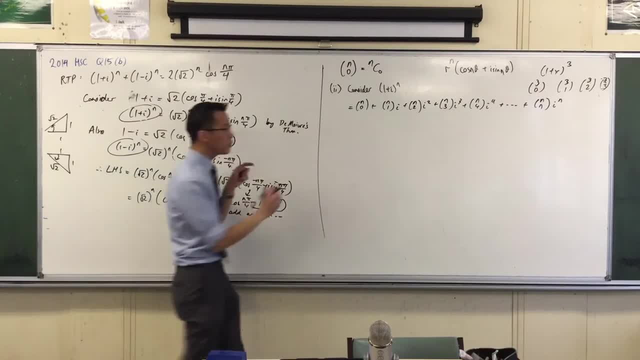 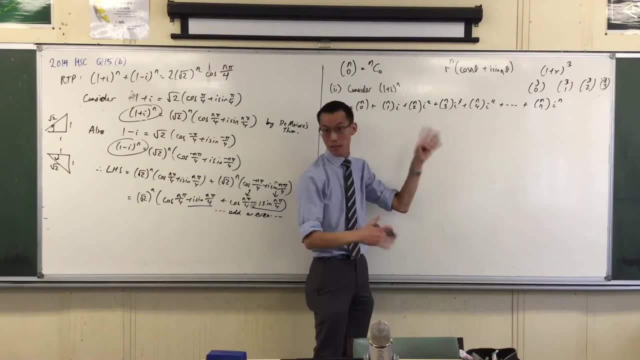 And whatever that happens to be, Okay. now I can do a little more work on this before I leave it and think about the other one. It's conjugate, Okay. Um, there's a whole bunch of i's here that can be cancelled out. 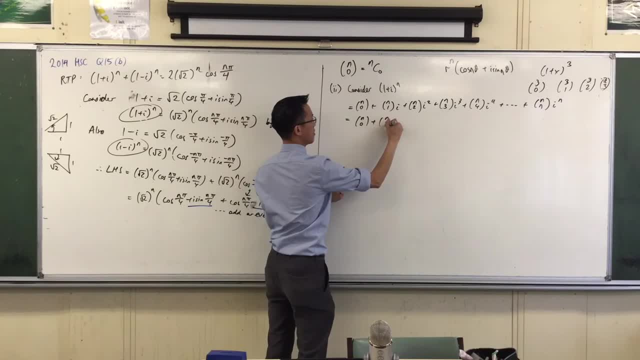 Do you agree, Right? Uh, these first two, they just kind of sit there, Right, But what about the next one? So yeah, i squared by definition is minus 1, right, So that's kind of cool. 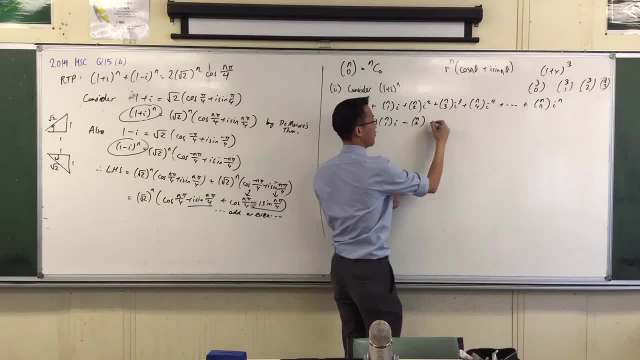 Now there's an i squared here as well, isn't there? So therefore it's minus, but there's still one i left over. Yeah, Yeah, Okay. Then I get to this one, Just plus 1.. And that's just plus 1, right. 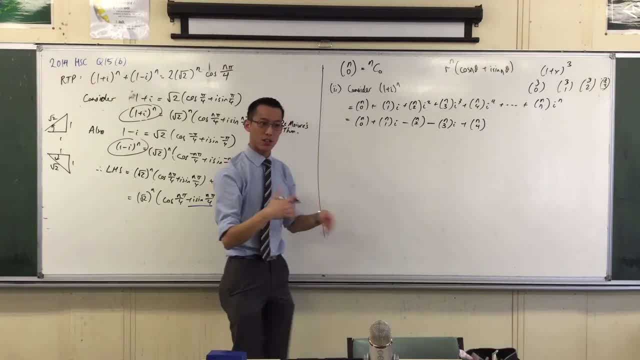 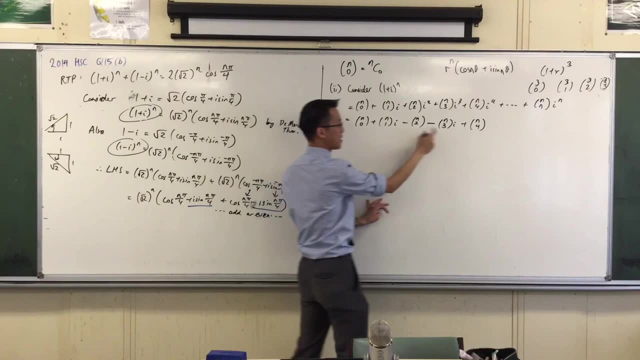 Do you see why I wrote a few extra terms now? Because usually 3 is enough to establish a pattern, but here the pattern takes longer It goes. look at the signs: Plus plus, Minus, minus, Right, No, i, i. 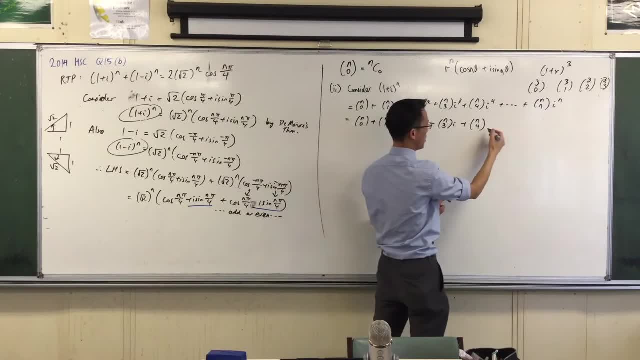 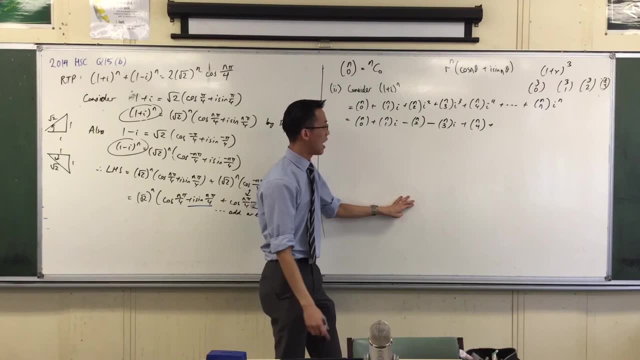 No, i, i And so on. Okay, The next one. What would the next one be? It's going to be plus. if I were to write it down, I think it would be plus Plus n 5 i, n 5, i. 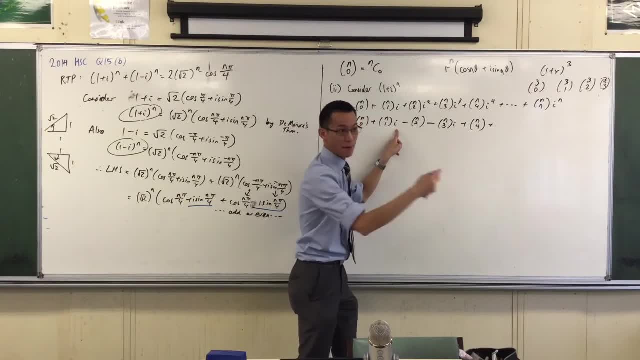 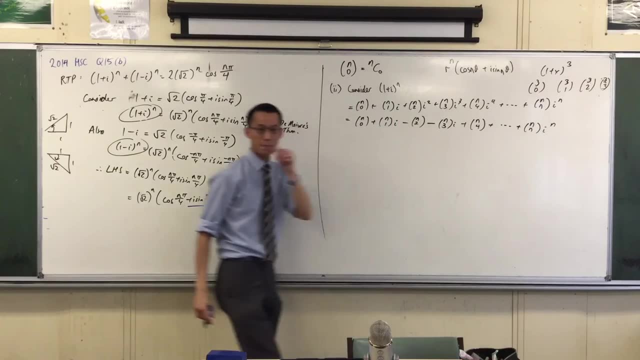 Yeah, Right, Because there's actually 5. i's there, but 4 of them have just sort of collapsed into 1.. Dot dot dot, Plus That. You okay with that? Okay, Now there's actually one more thing I can do to this. 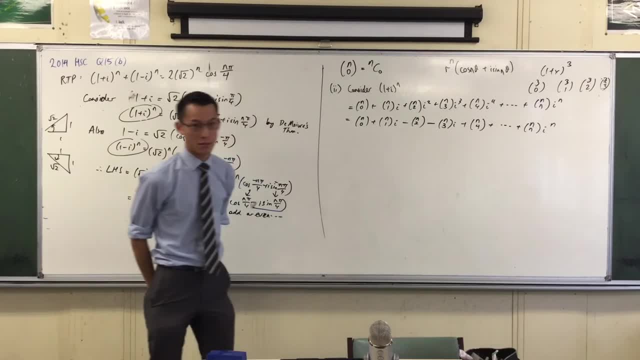 There's one more thing I can do to this n What's n? Look at the question again. Yeah, n is not just anything. n is divisible by 4. 4.. 1,, 2, 3.. Sorry. 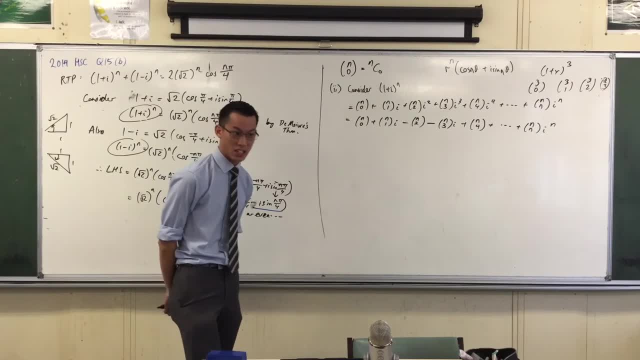 1,, 2,, 3,, 4.. Right, And then 1,, 2,, 3,, 4.. And then 1,, 2,, 3,, 4.. And then eventually this guy.